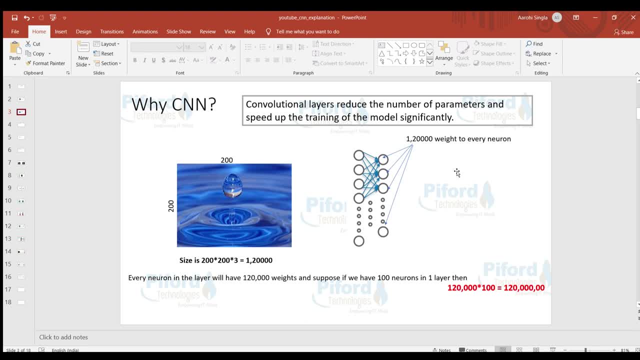 networks. what are the disadvantage of fully connected network and why we need CNN. Let's understand that. So let's refer this picture for this. So this image is of 200 by 200 and this is a colored image, So that means 200 into 200 into. 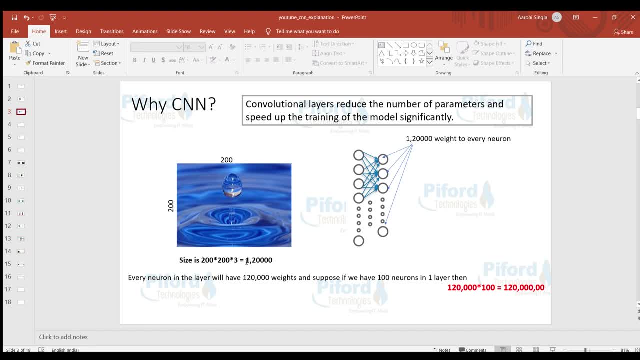 3. So if you multiply this value we'll get 1 lakh 20,000 weights, right? So that simply means if we are using fully connected network, that means every neuron will have these many weights. And suppose if we have 100 neurons in one layer, then means: 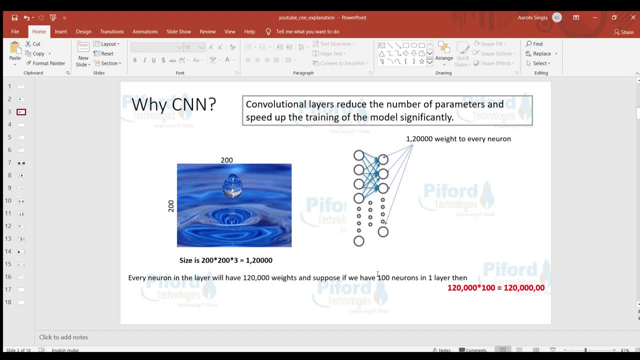 if we have 100 neurons in one layer, that simply means every neuron will have these many weights. That means multiply this 1 lakh 20,000 weight into 100 neurons and we'll be having these many neurons. So fully connected network is fully based over here, right, And why we need CNN. 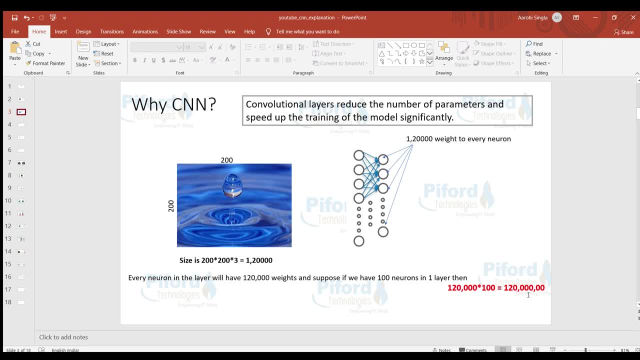 Because in CNN neuron in a layer will only be connected to a small region of the layer instead of, you know, all the neurons in a fully connected layer. So CNN is basically a partial connected network. So if you'll see this network over here, 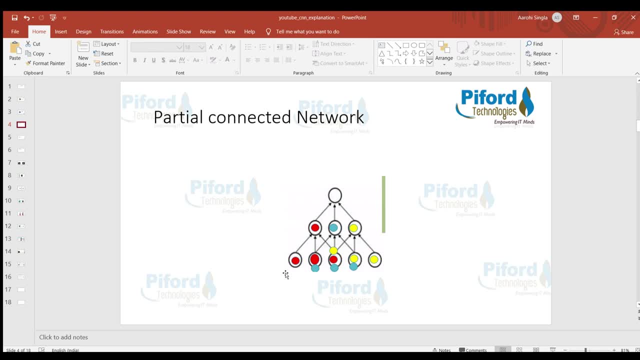 first neuron, red neuron, is only connected to the three neurons, instead of five neurons. See, instead of these five neurons, this red neuron is only connected to the three neurons, And in the same way blue and yellow neuron does right. So basically, CNN layers reduce the number. 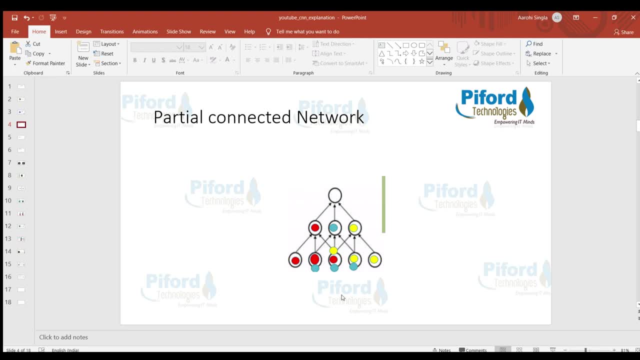 of parameters and speed up the training of the model Right. So there are three types of layers in convolutional neural network. First layer is convolutional layer, second layer is relu layer and third layer is pooling layer. Let's discuss each and every layer one by one, with proper explanation. 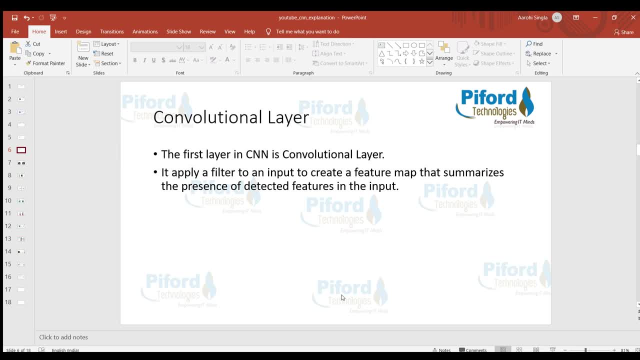 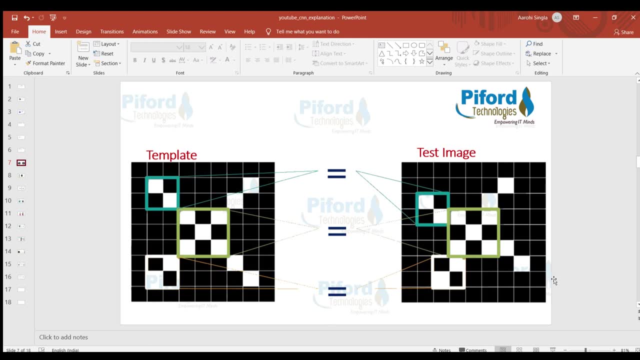 So the first layer is in CNN, is convolutional layer. What is the work of convolutional layer? Let's understand this. So, to understand the work of convolutional layer, we will, you know, see this image. This is a template and this is the test image, Right? So suppose we have created? 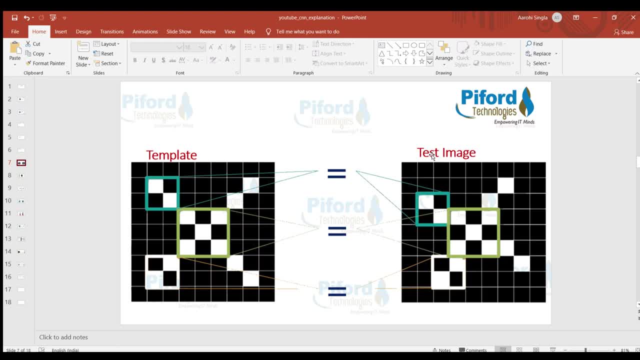 a classifier which should classify the image. Right Means, if the input image which we are giving to our algorithm is X, then our algorithm, should, you know, classify that image as X. In the same way, if we give any other alphabet, then our algorithm should be capable to detect. 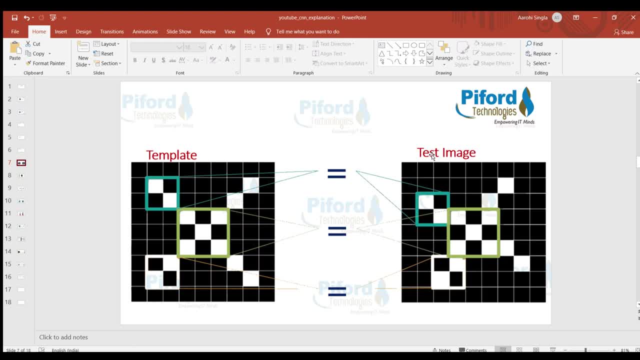 whether that particular image belongs to which particular Alphabet Right. So here the test image is of X. So this is the image. So this is the test image of X, But it is a distorted image. Right, Distorted image means it is not exactly at the same position. 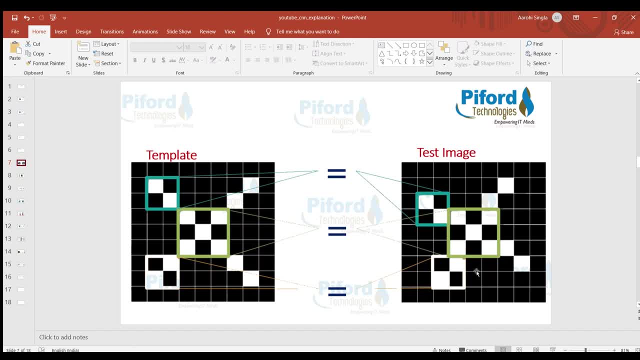 but roughly at the same position Means, if you will compare this image with this perfect template. So we know like this is the image of X only, but the pixels are not exactly at same position, but roughly at same position. All right, 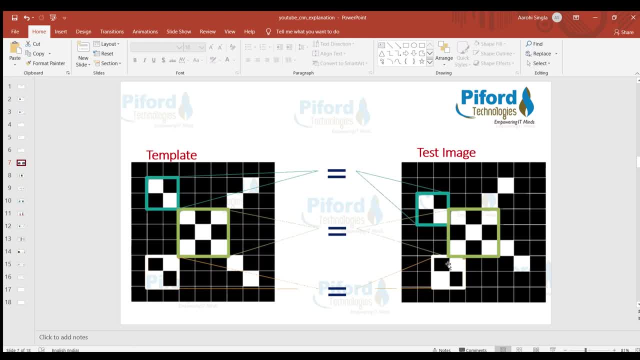 So how CNN work. So, as I have told you, the very first layer is convolutional layer. So the task of convolutional layer is to divide the image into features. So these are the features. This is one feature- 2 by 2, which is the size of 2 by 2.. Here we have a feature of 3 by 3 and here 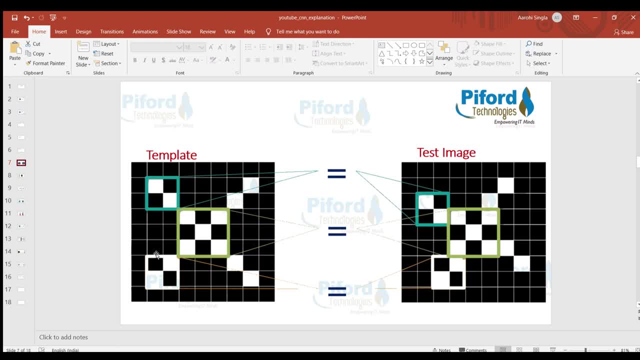 we have a feature of 2 by 2.. So CNN splits the image into features and in this image we have three features Right And then it tries to see these features are available in test image or not. Means firstly we divided our image into features. Then it will check whether this particular 2 by 2 feature is. 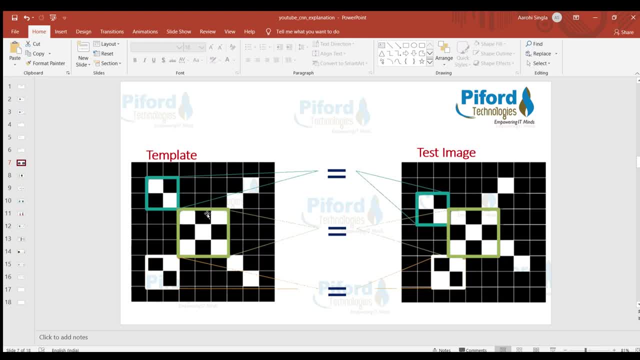 available in this test image, And then it will check whether this 3 by 3 feature is available in this test image. In the same way, it will look for other features also. So let's see the pattern 2 by 2.. The very first pattern is 2 by 2.. Right, So it will see that this pattern matching in the 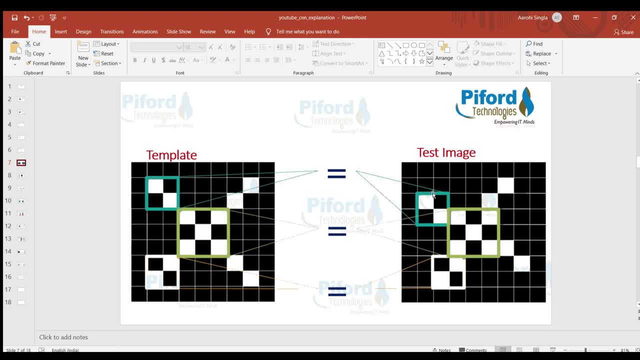 test image or not. So, as we can see, this pattern is matching over here. The pixels are not exactly at same position, Right? But with the feature, this feature is over here also and we have this feature over here also- Then obviously our algorithm will know: like, okay, this feature. 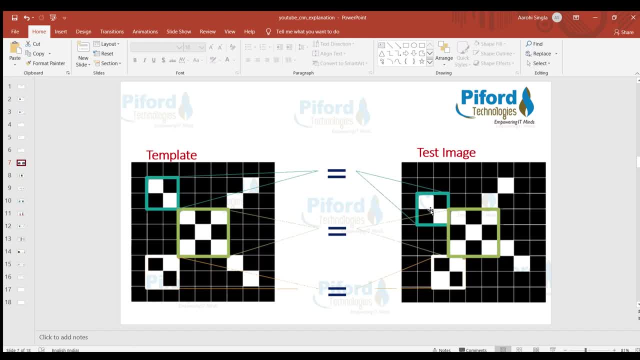 is available in test image also. So basically, what I'm trying to say is: CNN does not match pixel to pixel pattern Right, Rather than it matches with the features. It does not match pixel to pixel. It matches with the features which we have created. It will see these features. 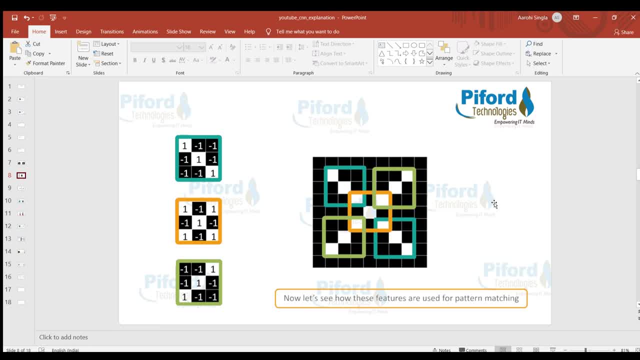 in the test image. So, as I have shown you, these are the 3 features. So it will check all these 3 features one by one in the test image So we can see this feature is available here and here in this image And this feature is available over here And this feature is available. 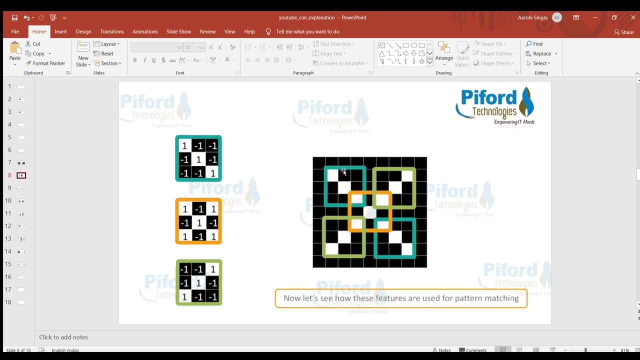 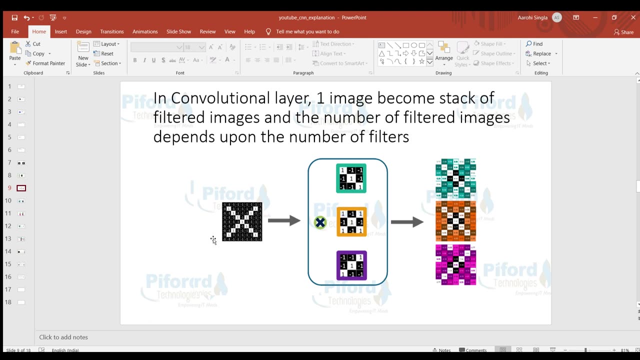 here and here and finally we see, this is the task of convolutional layer. the very first layer of convolutional neural network is convolutional layer, whose task is, whose task is to create filters. so this is our image and on this image, the very first layer is convolutional layer. so 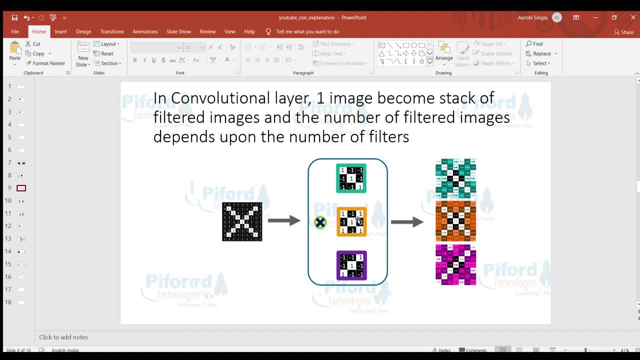 this is a symbol of convolutional layer. so when- and these are the three features which we have decided on, this feature in this image- right so when we convolve these features, these filters, with this image, we get these three images- means the output of this convolutional layer is this: 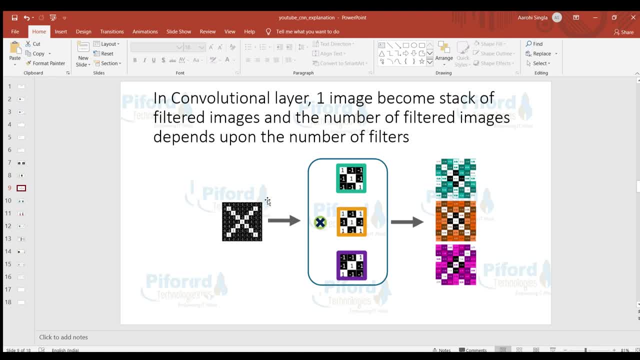 input to convolutional layer is this, and when we applied three filters on it, we get three filtered images. right, so these are the stack of images you so. output of convolutional layer is stack of filtered images. means when we convolve these three features on the input image, we get three filtered images, and these filtered images depends. 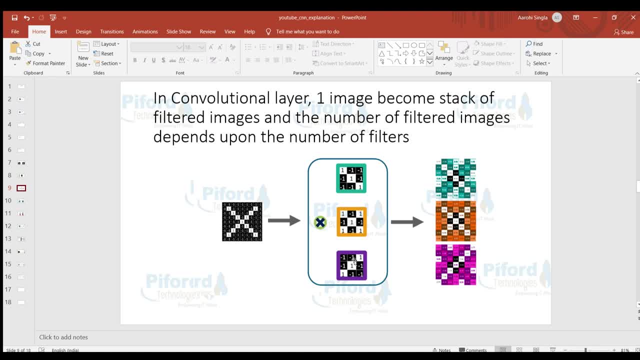 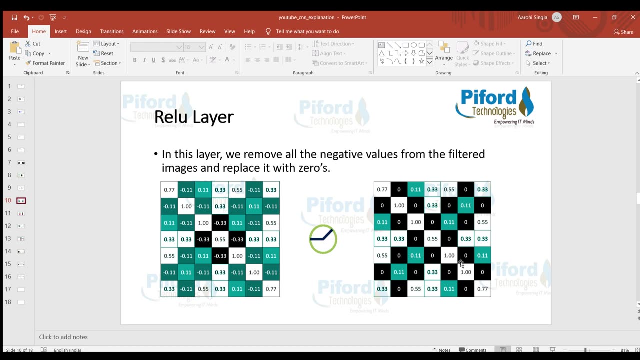 upon the number of filters we are applying over here. suppose, if we apply five filters over here, then how many filter images will get? five filtered images will get. so this is the output of filtered convolutional layer. so the next layer is inside the folder twin pełner. it contains zero filters and the second filter image. it contains 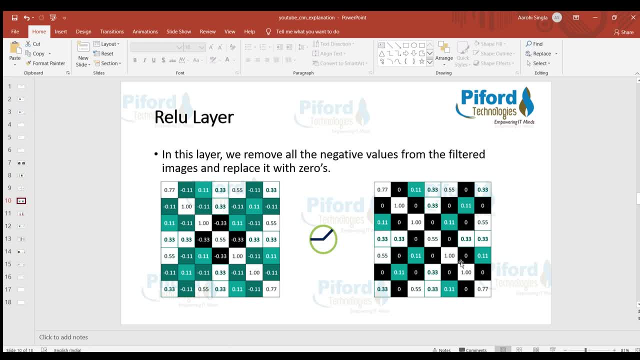 only one filter image. this filter image you can see here. this is only one filter in words. so if you go on your android laptop and you go and take a look at this encounter mode, let me give you guys adem werei 19, which is the reverse load. Kookaburra grants us zero. 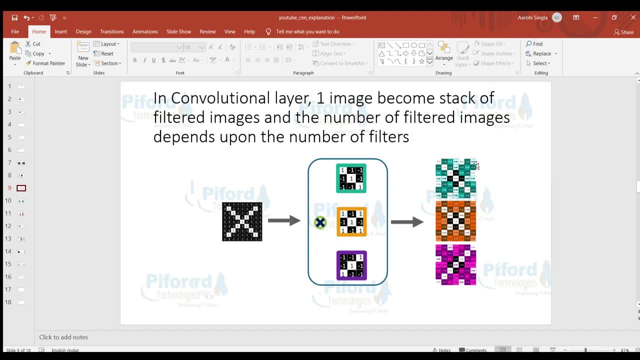 filters which are centered as a higher order filter image and we require a multiple filter image, right, and we are taking a look at the number of filters that we are using here. this is a filter image, this is a layered filter image, this is二 filter image and this is trois filter image. this two filter images. 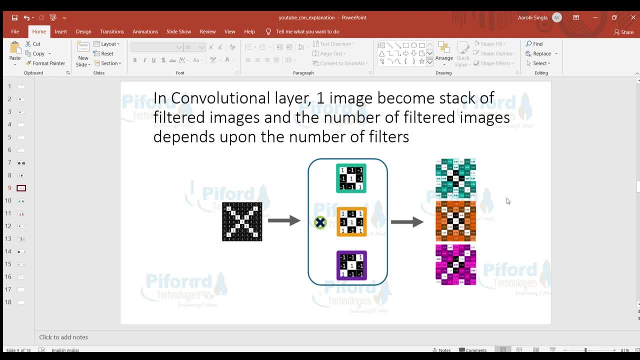 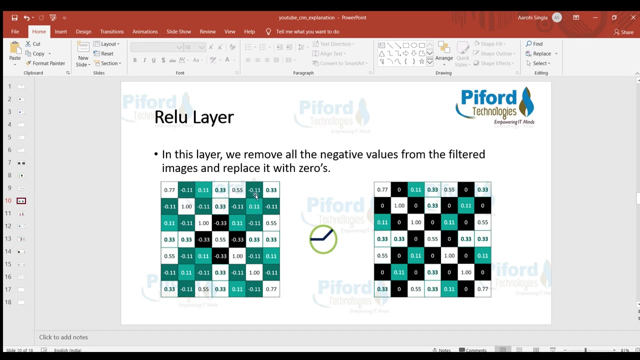 image. So on these three filtered images, we'll apply that ReLU function one by one. So I'm showing you first of all, I'm showing you the example with the first filtered image. So this is the first filtered image. So you'll see here the second record minus 0.11 right, and then this: 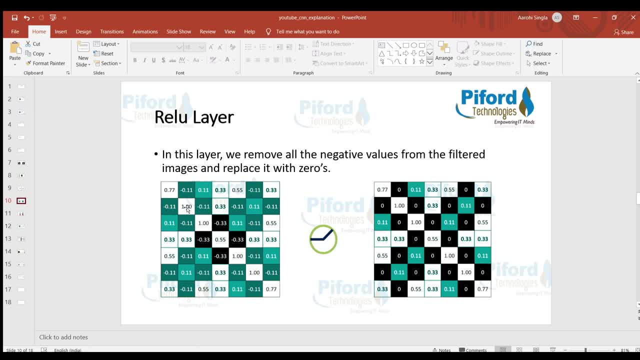 is again a negative record over here. this is again a negative record. So when we applied- this is a symbol of ReLU layer- when we applied ReLU on this filtered image, we get this kind of output. So you'll see all the negative values get replaced by 0. So in the same way, we perform ReLU on three. 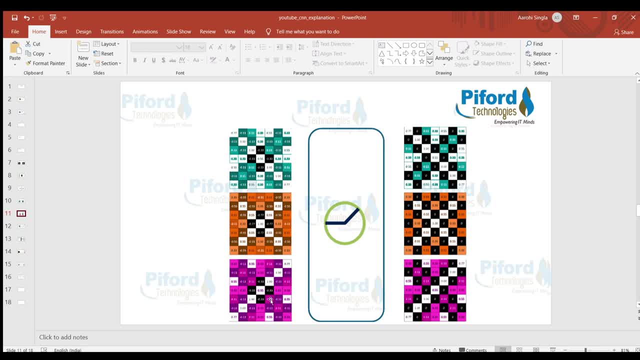 of the filtered images. So these are the filtered images after convolutional layer. When we apply ReLU on it, we get these three filtered images right. So what we does over here? we simply applied ReLU function Which converted all the negative images into 0. Then the next layer is pooling layer. Now what is? 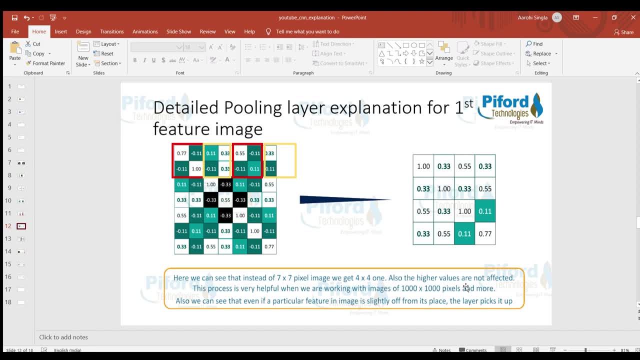 pooling layer. See, the ultimate goal of pooling layer is to reduce the size of image. So over here the size of image is. over here, if you'll see, the size of image is 7 by 7.. 1,, 2,, 3,, 4,, 5,, 6, 7.. 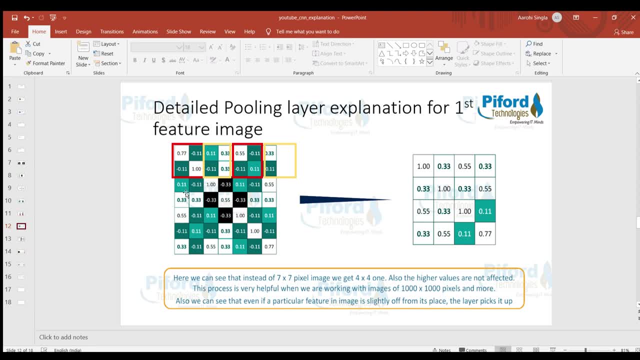 7 rows and 7 columns we have. The size of image is 7 by 7, and when we applied ReLU on it, we get this kind of output. So this is the ultimate goal of pooling layer. So over here, pooling on it. So this is a symbol of pooling. When we applied pooling on it, we get 1,, 2,, 3,, 4,. 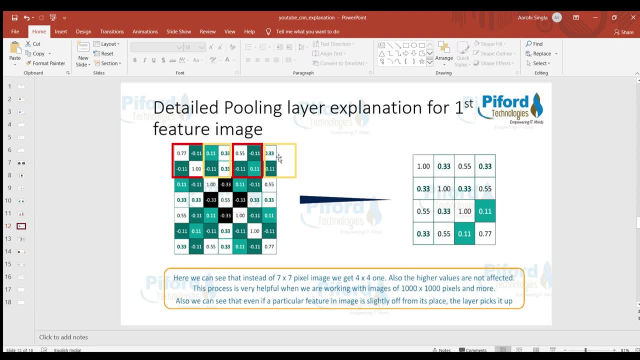 4 by 4 image Means from 7 by 7 image, our image get shrinked to 4 by 4.. So how to do this? See, the very first step is to pick a window size. So if you see here, so this is a window size, This is one window. 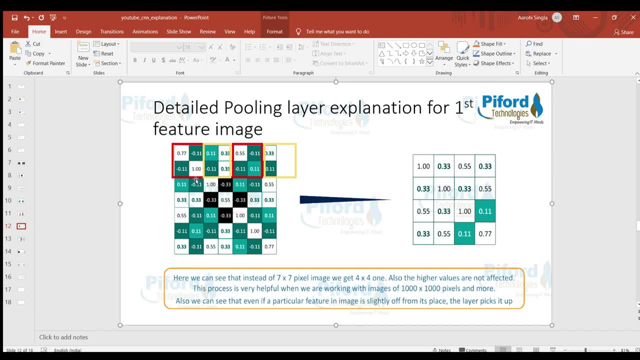 this is two window. The window size I've chosen over here is 2 by 2.. 2 this side and 2 by this side. So this is the first window. So once you choose the window, we need to find out which is the highest value from that window. So if 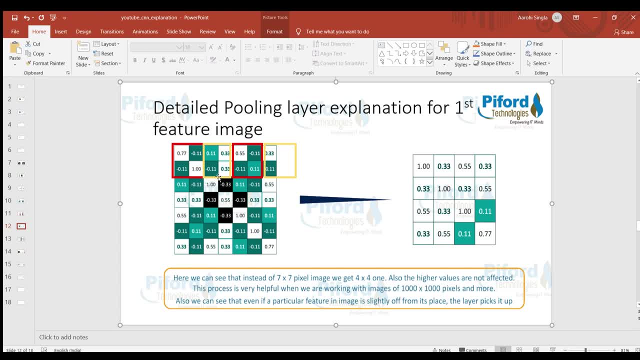 you'll see all these four value. this one is the highest value, So we'll pick one and we'll, you know, put that one over here In the same way then, okay, this is a 2 by 2 window. then we need to choose a stride also. Stride simply means how much we want to shift it to the right side and how much. 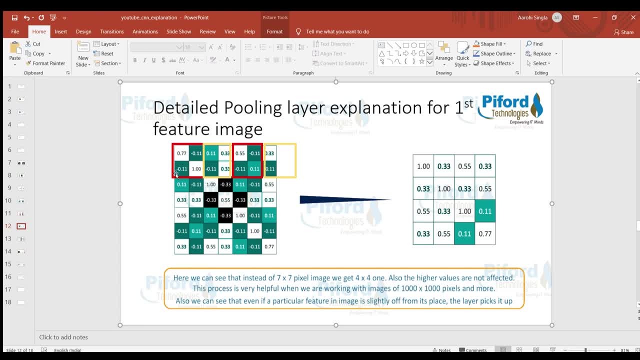 shift. we want on Downward side. So this is a 2 by 2 window. We are shifting. Stride is 2 over here. That means jump of 2, and this is the next window. Now, from this yellow window, choose which is the highest value, Fill that. 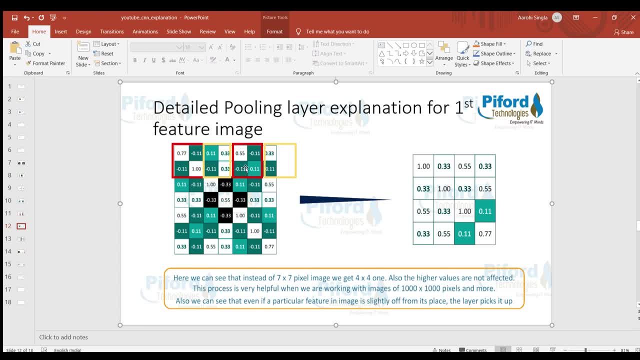 value over here. and then this is the third window- Choose the highest value from here and fill it over here. and in the fourth window we are not having two values. then we can simply choose between these two. which is the highest value? So 0.33 is the highest value. 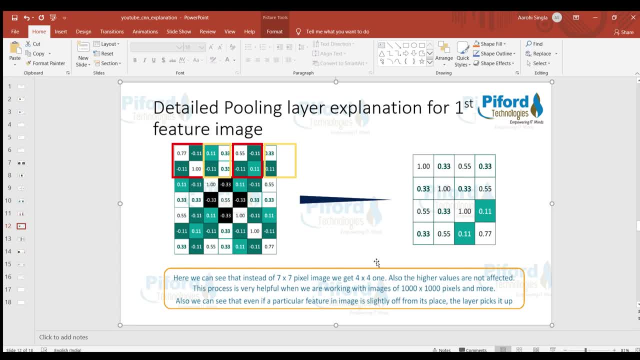 We'll write it over here In the same way. this process will, you know, go along. So what we does over here: first we pick the window size, We choose the stride, and then we pass the window across the filtered images and from each window we are picking the value which has maximum number, Right? So this? 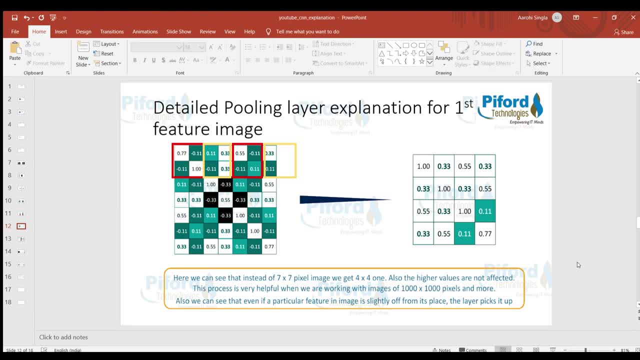 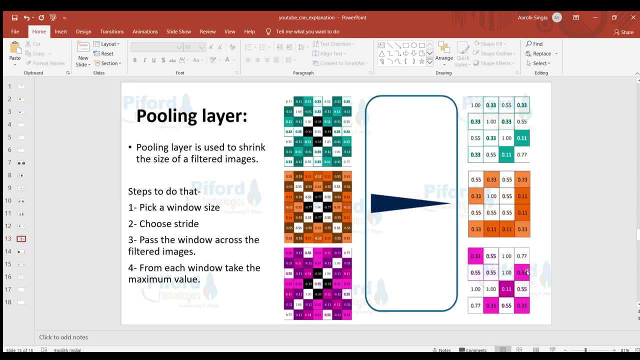 is how pooling layer work. So now I've shown you How convolutional layer, ReLU layer and pooling layer work. Now this is the pooling task I have done on all the three filtered images. These are the filtered images, Right? So on these three filtered images, I have applied pooling and now I 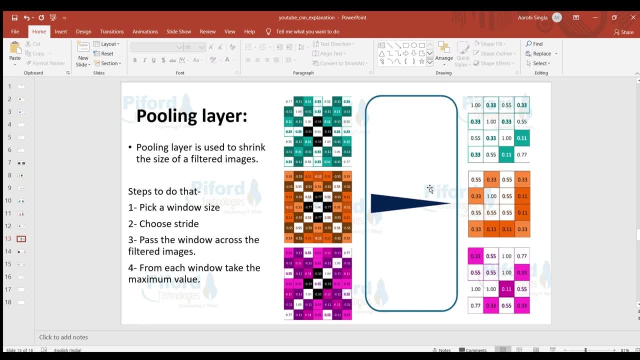 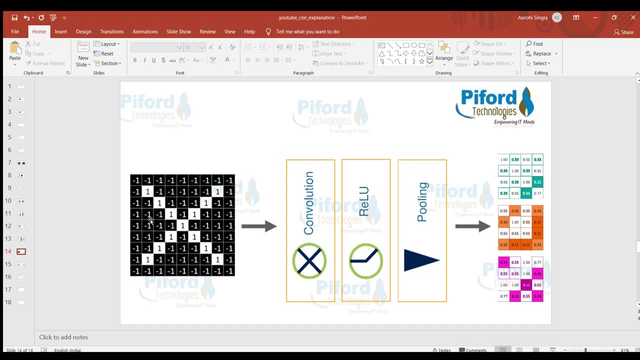 have 4 by 4 of image filtered images, Right? So this is how the whole process looks like. So this is. this was the image input image. This input image we gave to convolutional network, then convolutional network applied filters on it, and then we used ReLU. ReLU deleted all, replaced all the negative values with 0s, and then we have pooling, layer pooling. 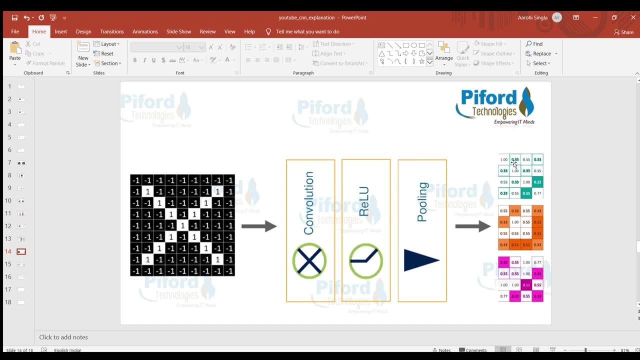 layer. What pooling layer does? It? shrinks the image size. and finally we have these three filtered images from the convolutional network. So right now we have 4 by 4 image. So sometimes, let's suppose, if you're working on images which have bigger size, then 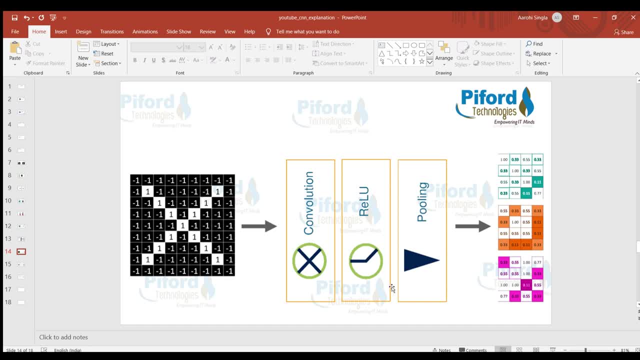 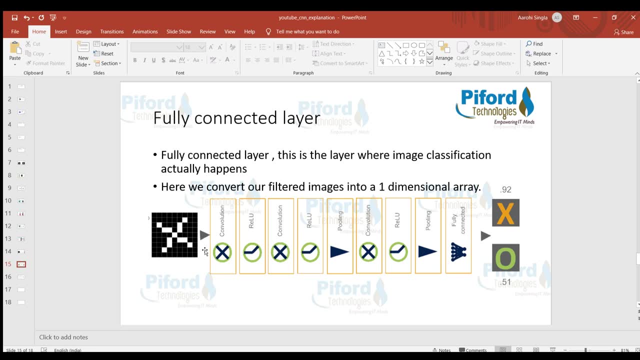 sometimes it is required. We need to run this convolutional ReLU and pooling layer. You might have used more of the pooling layer, So now let's run this convolutional ReLU and pooling layer multiple times. Let me show you how. Suppose this is the image on which I want to work. 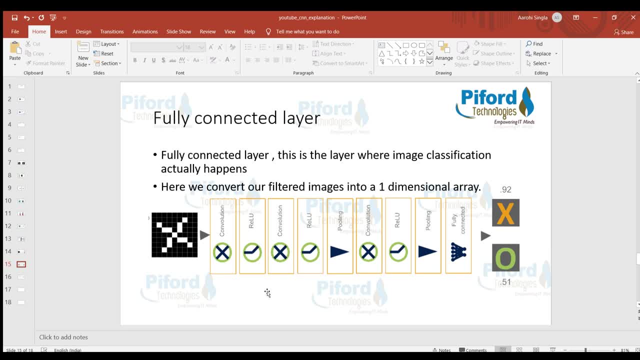 See. Yes, this is the symbol of convolutional layer and the pooling layer. So again convolutional ReLU and then pooling layer, then again convolutional ReLU and pooling. So this is the process, See, I have used over here. 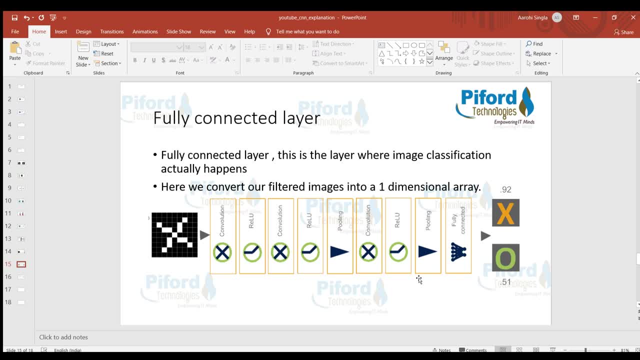 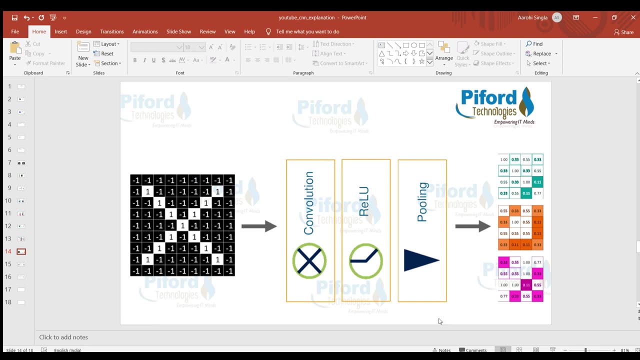 convolutional ReLU multiple times and finally. finally, when you want to classify whether this image is of which particular alphabet, then you need to convert your filtered images. see the output of this convolutional neural network would be like this, but when we want to perform the classification, 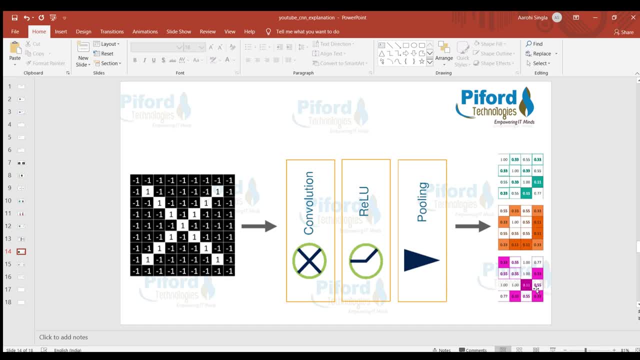 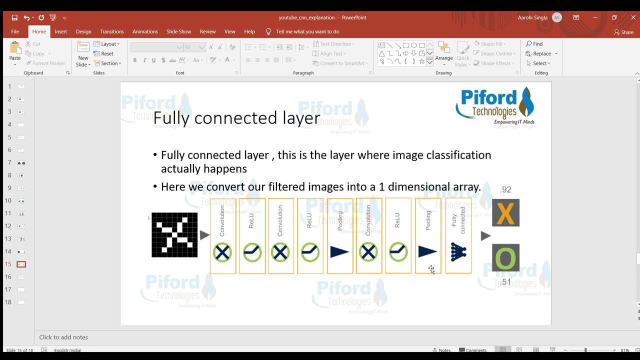 on it, then we need to convert these two-dimensional images into one-dimensional array. so this is what we are doing over here, so we are converting our this images into one-dimensional array and then we are giving it to fully connected layer, right? so then, finally, it will tell us: 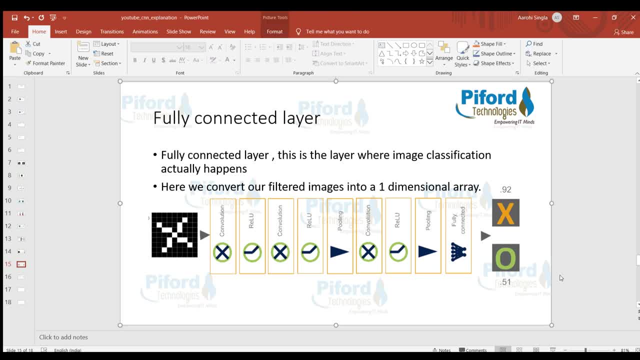 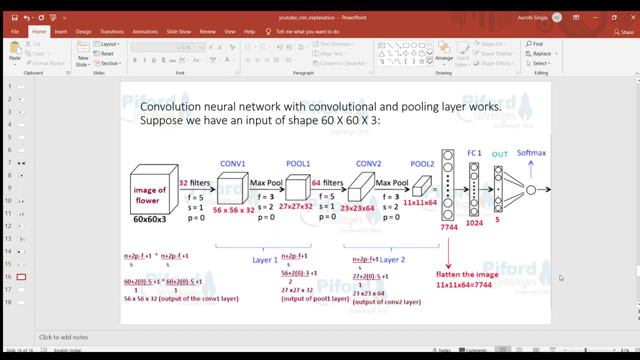 whether this particular image is of which particular you know, object or class- so clear. so now let me show you the process, like how to choose number of filters, how different side values are working, what is the padding and what is how pooling layer is working, how the image size is getting reduced. let's discuss that with the help of this image. so 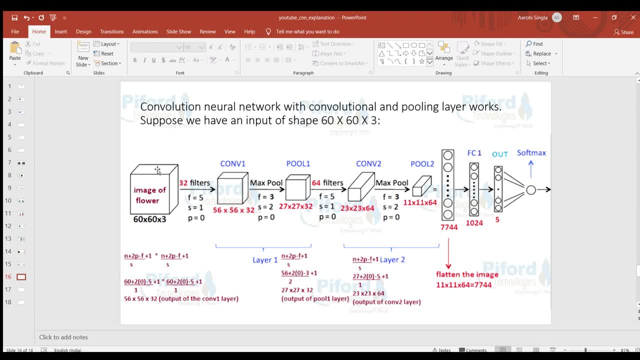 initially, we have an image, suppose this image is a flower and the size of this image is 60 into 60 into 3. so this 3 means this is a colored image and this is the height and width of the image, right. so now this image. i want to give this image to a convolutional layer. 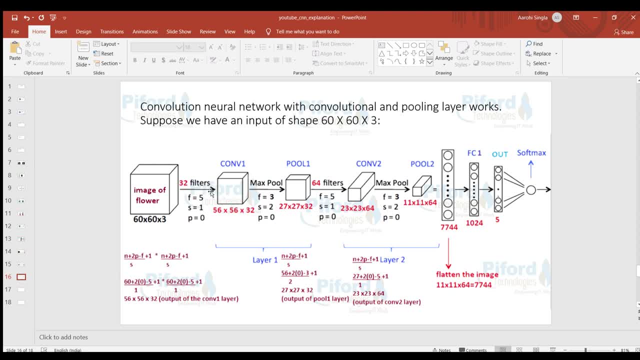 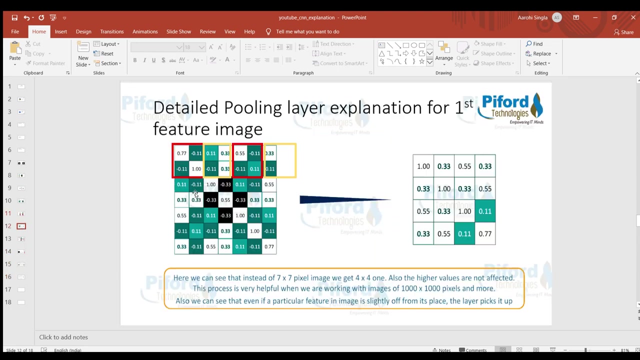 so this is the first convolutional layer. so in cnn network the very first layer is convolutional layer. so this is the convolutional layer. so what we are doing over here is i'm saying i want to apply 32 filters, right, and the filter size should be 5 by 5. so remember here, let me 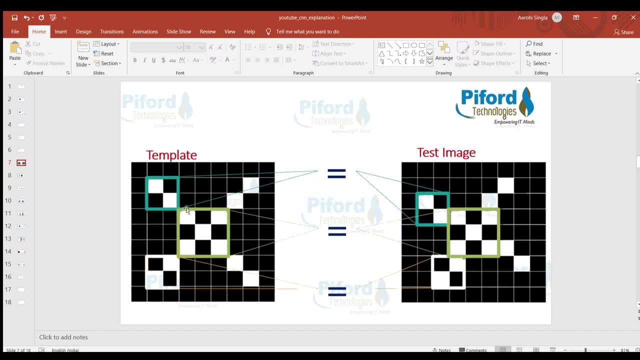 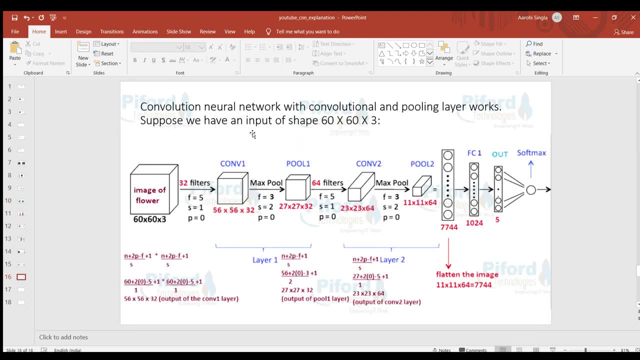 tell you over here we have three filters, and two filters have size of 2 by 2 and one filter is of 3 by 3 size. in the same way, i'm saying over here: i want 32 filters on this image and filter size should be 5 by 5 and sprite should be 1 and padding. 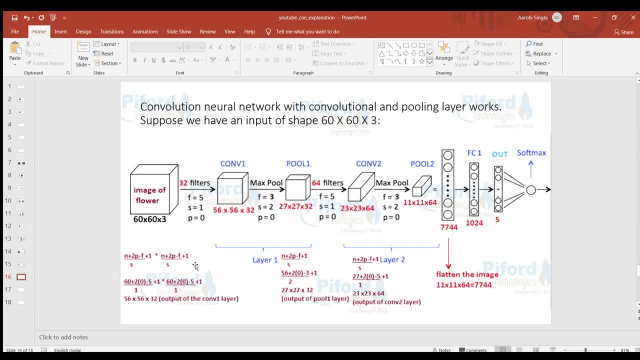 should be 0. now see, this is the formula which get applied and we'll get the output. so the formula is n plus 2p minus f by s plus 1 into n plus 2p minus f by s plus 1. so n. is this the image size, the actual image size, 60 plus 2? what? 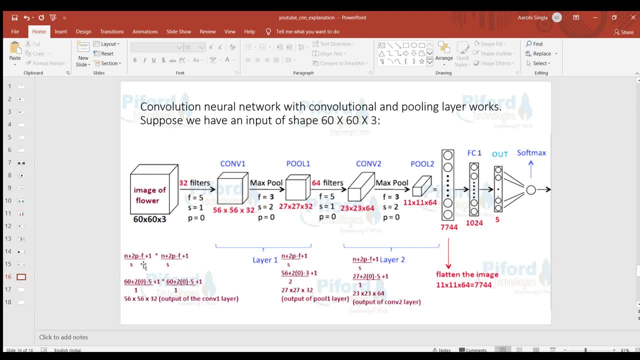 is padding over here 0, so we put 0 over here. and this f is how many filter, the filter size. so the filter size is 5 by 5, so we are writing 5 over here. stride is 1, so s 1 over here. in the same way, 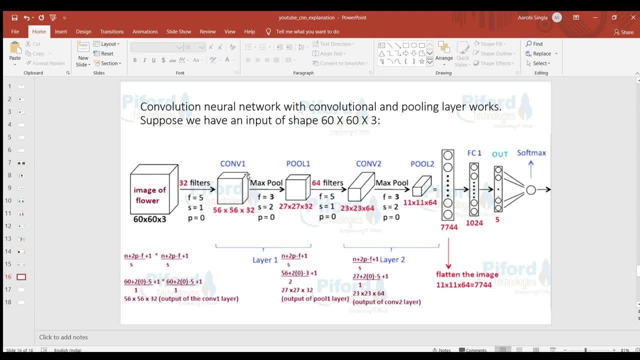 applied on this way. so the output of this convolutional layer would be 56 into 56 into 32 means the output of this convolutional layer when we apply 32 filters on it with filter size of 5 by 5 and strate 1 and padding 0, we will be getting this output. 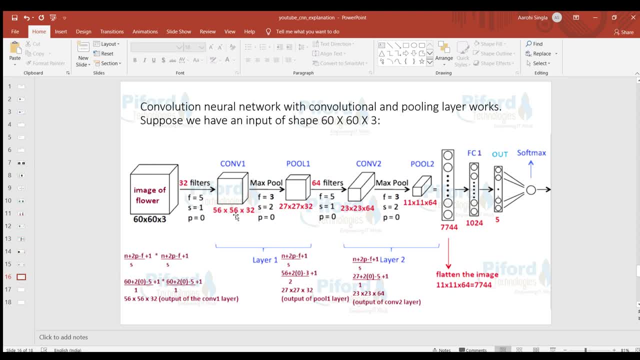 means image size gets reduced to 56 by 56. and see- this is the important thing to notice over here- what we are having. all these filters, your drawing fill, and see, this is the important thing to notice over here- what we are having over here is the fade. 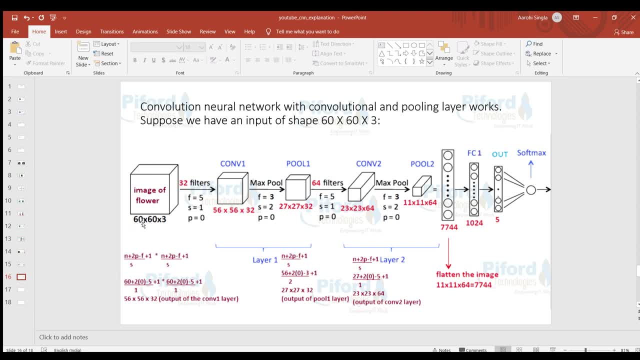 the fade. and now what our model would say that over here- so that's where we are getting this other layer over here, that's veraj, and what we are getting over here is 32 and 60 by 60, by what we are having over here is 3, so we all know. 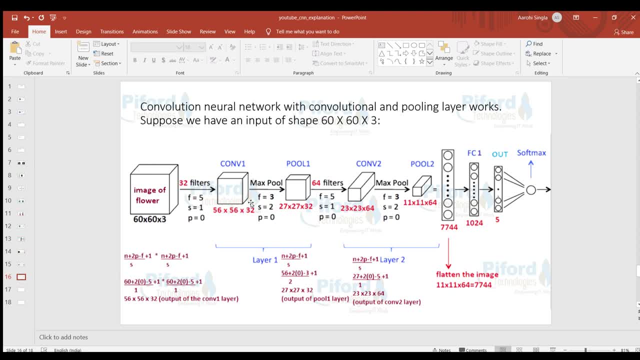 this 3 means we are talking about colored images, but why we are having 32 over here? so we are having 32 over here because we are having 32 filter. so if you remember from my today class only, as I've told you, let me show you once again. 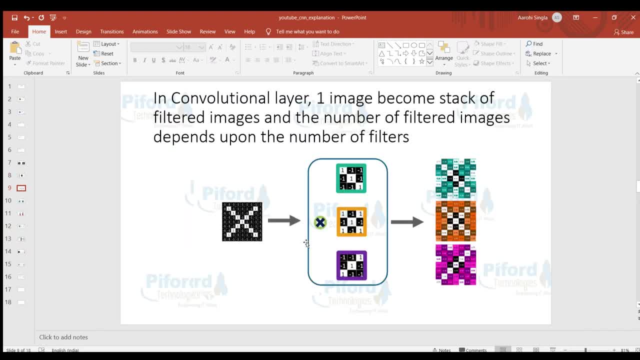 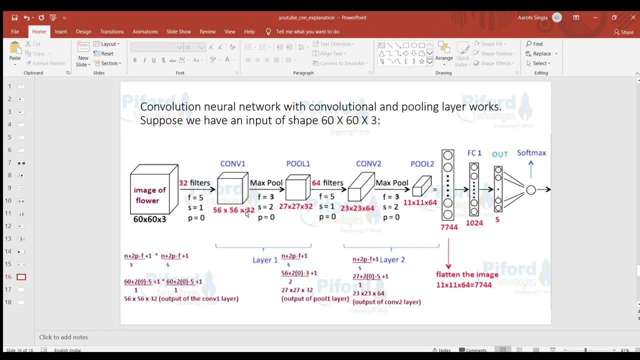 over here. see, we will be getting number of filtered images, and how many filtered images will be getting it depends upon the number of filters we are applying, right? so this is what we are doing over here. so how many filters we are applying: 32. so that means we are getting 32 filtered images and every filtered 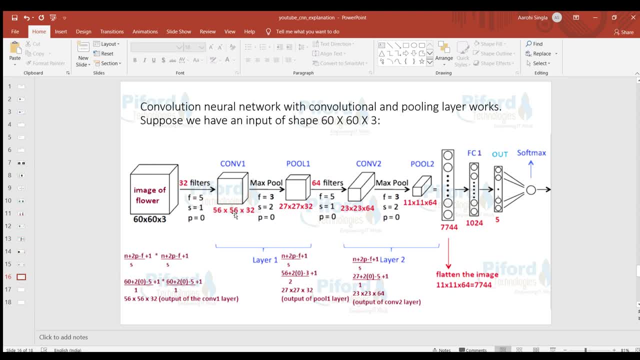 images would be. every filtered image would be of 56 by 56, and we have 32 such filtered images right. so now this is the output of convolutional layer. now we have pooling layer right now. see, if you'll see, I'm not using ReLU over here, so it is not always necessary. see, it depends upon the type. 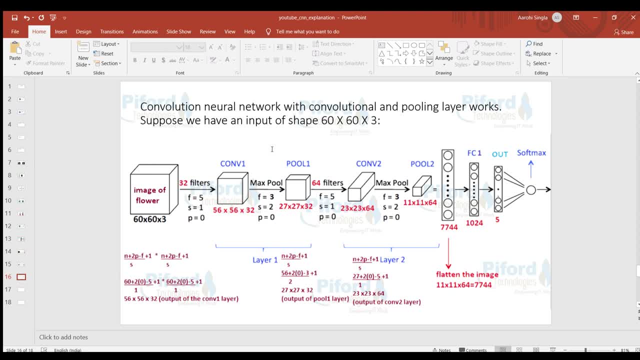 of image and your problem type, like whether to choose ReLU or not right now. right. so if you want, you can choose ReLU over here. but I am straight away using here pooling layer, right? so the output of the previous layer will become the input of next layer. so the output of convolutional layer is 56. 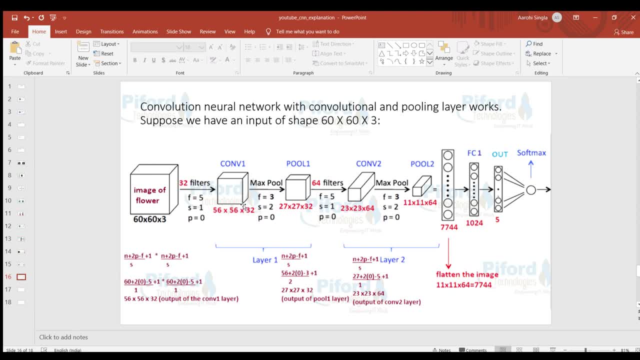 by 56 into 32 means we have 32 filtered images of 56 by 56. we are giving this input to max pool. so if you remember from pooling layer what we does in pooling layer, let me show you again what we does in pooling layer. we 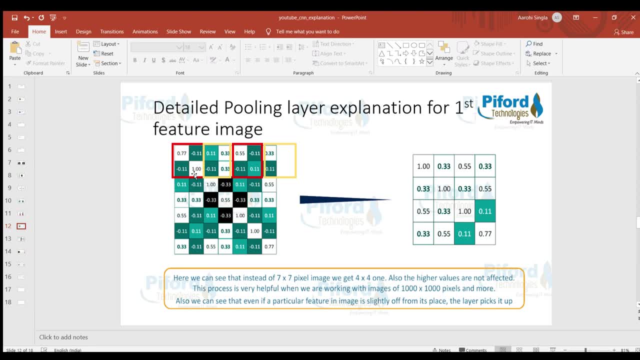 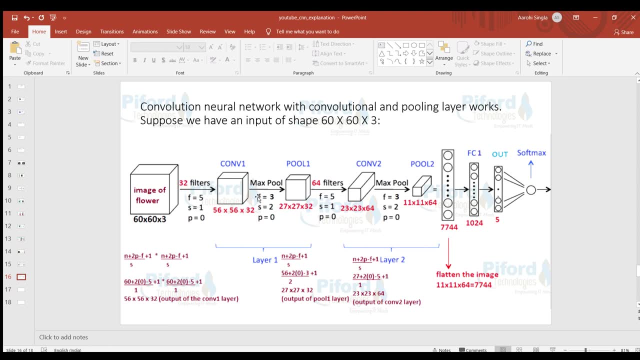 choose a window size and then, finally, we choose the highest value from that window, right? so this is what I'm doing over here. so over here I'm saying: window size is, F, is equal to three, means window size is three by three and stride is two and padding is zero. so see, the formula is: 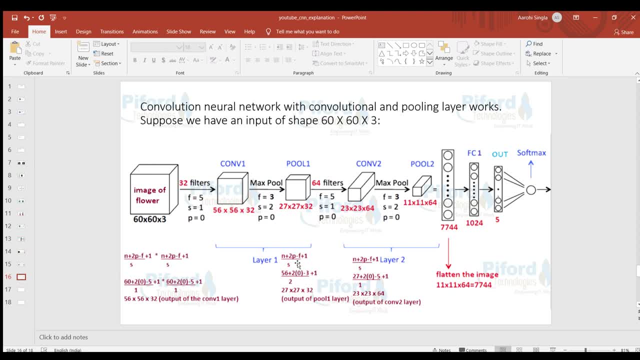 again same N plus 2, P minus F plus 1 by S. so what is N now the image size? image size is 56. in this case two padding is still zero. so is zero minus F. what is F over here? filter size means the window size is three and stride is. 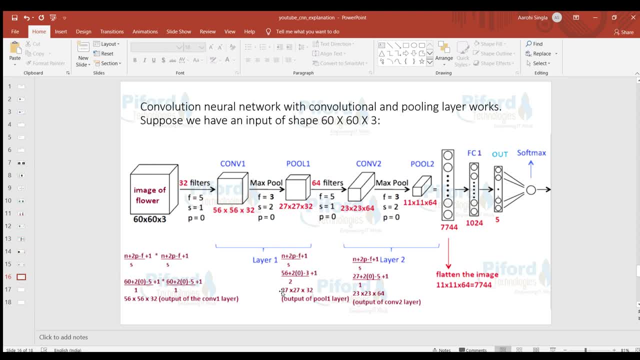 is 2, so when you'll apply this formula, so you'll get 27 by 27 into 27 into 27 into 32. so you'll see the output of this pooling layer is 27 by 27 into 32. previously our image is 56 by 56, now our 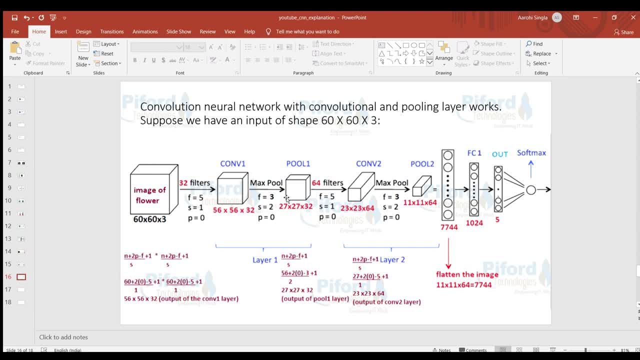 image got shrinked and we have our image of 27 by 27 and into 32, because we have 32 such images, filtered images, right? so this is how pooling layer reduce the size of image. okay, now again I see, and now we have image size of 27 by 27. now I still want to reduce the size of image. then I can. 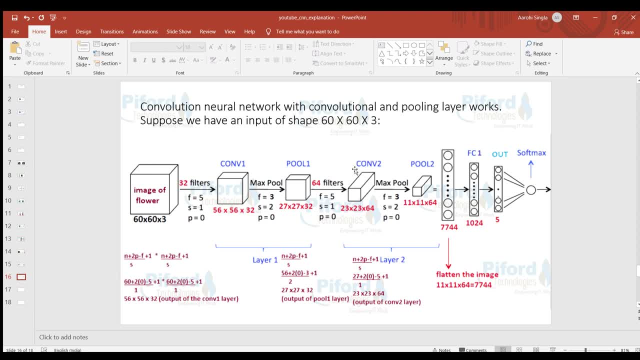 again apply convolutional layer. so this is again another convolutional layer over here. so this time what I'm doing is I'm saying: I want to apply 64 filters, right, and every filter should be of 5 by 5, with stride 1 and padding 0: same. apply the formula. right, when you'll apply the formula? 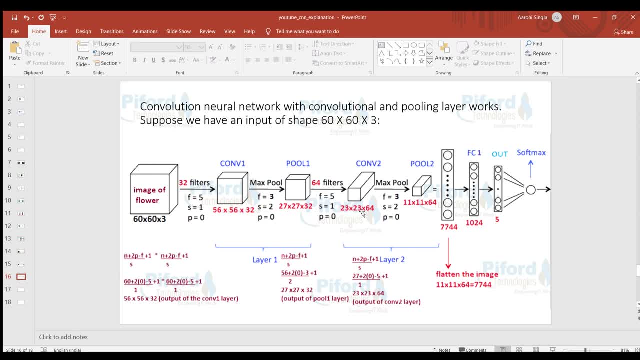 you'll get this output 23 by 23 into 64 now. see, now we have 64 over here. previously we were having 32. why we were having 32? because we were using 32 filters, but now we were using 64 filter, so we are going to have 64 filtered images of 23 by 23, now again using pooling layer on it. 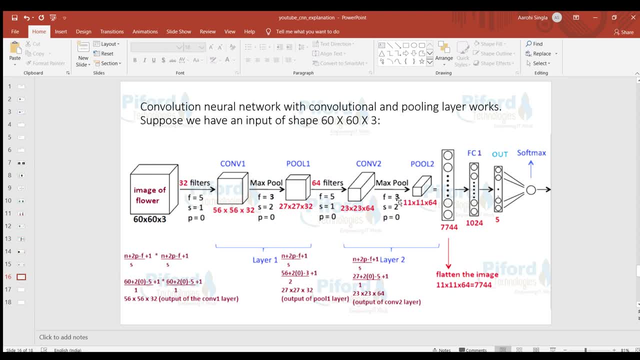 so again with the with pooling layer, Im saying filter size is 3 by 3, stride is 2 and padding is 0. again, apply the formula and you will get image of 11 by 11 into 64. means our actual image size is 60 by 60 into 3. but from this 60 by 60 image now we have an image of 11 by 11, right, and we have 64. 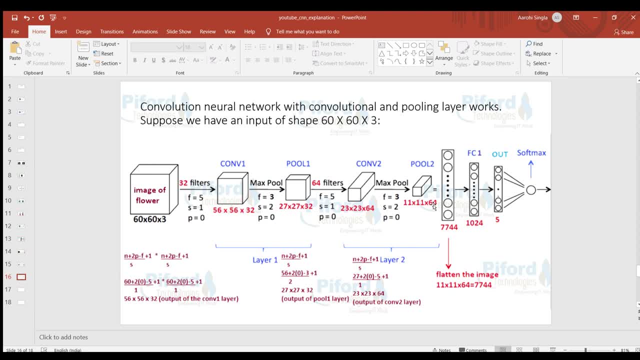 such filtered images. so, as I showed you, the image size was 84 by 3 divided by 1, and the wünsche limit is 0, told you few minutes back only that, when this is the this, we have, you know, processed our image, but now if we want to apply a classifier on it, then we need to convert these images into a. 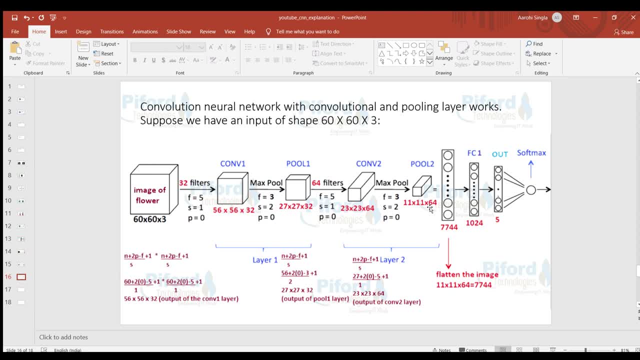 one-dimensional image. so multiply 11 into 11 into 64, so we'll get 7744 right. and then I'm giving these value to a fully connected layer and we have 1024 neurons in it. and finally I have output layer and we have a software function which is predicting the output. see, this is how convolutional. 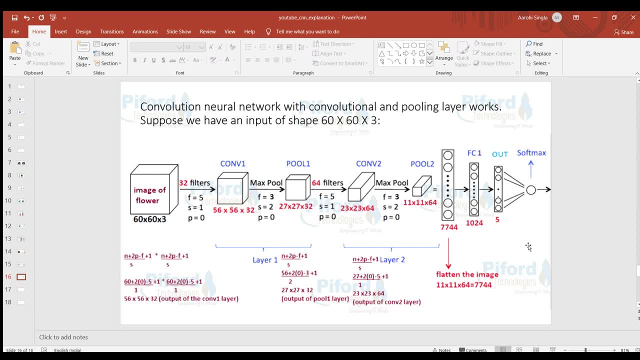 neural network work. the only thing which we need to take care is CNN have three layers: convolutional layer, ReLU layer and pooling layer. Convolutional layer is responsible for deciding the number of features, number of filters, and then we have ReLU layer, which will delete, replace all the negative values with 0, and then we have 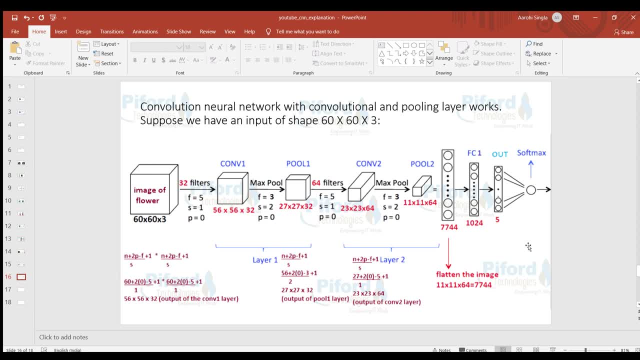 pooling layer. the task of pooling layer is to reduce the size of image, right, thank you.